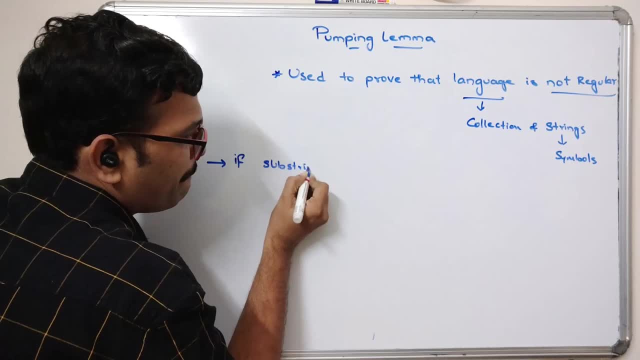 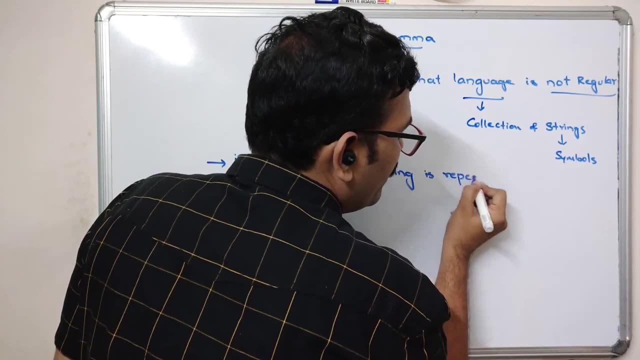 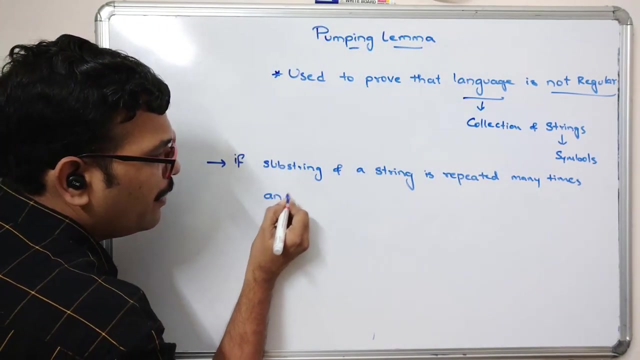 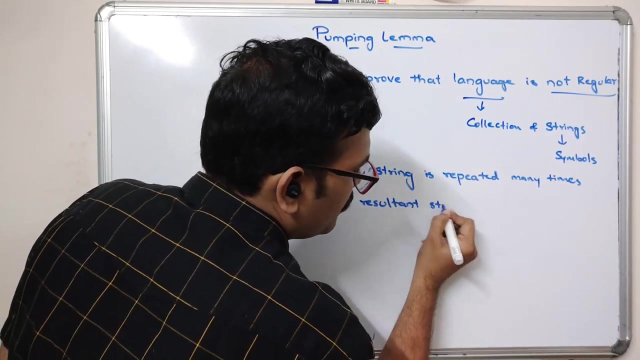 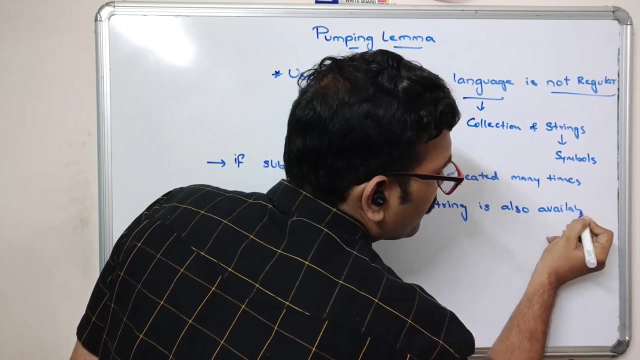 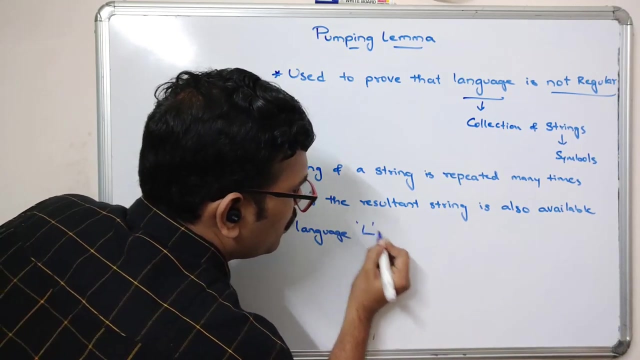 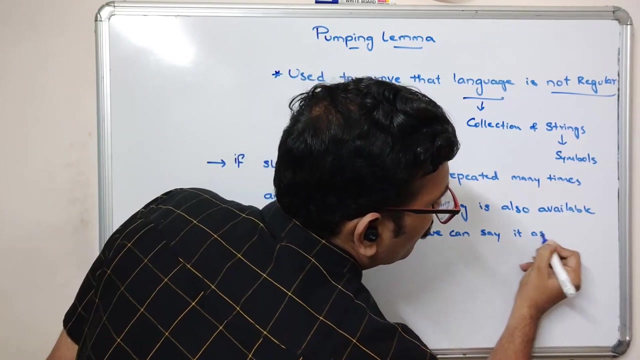 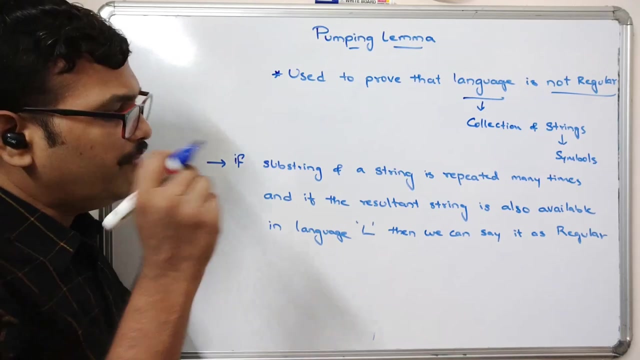 the substring. substring of a string is repeated many times and if the resultant string is also available, Okay, in language L, then we can say it as regular. So we know that the language will be having different strings, right? So if you consider any string and if the substring of that particular 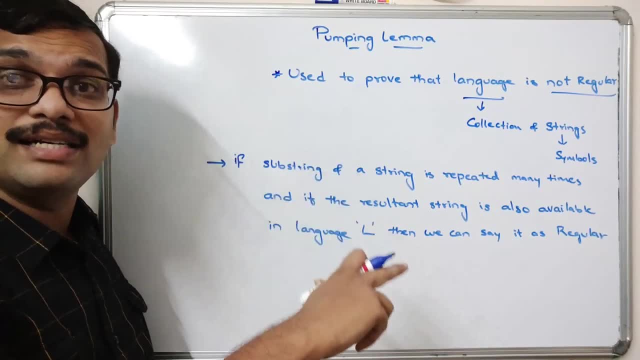 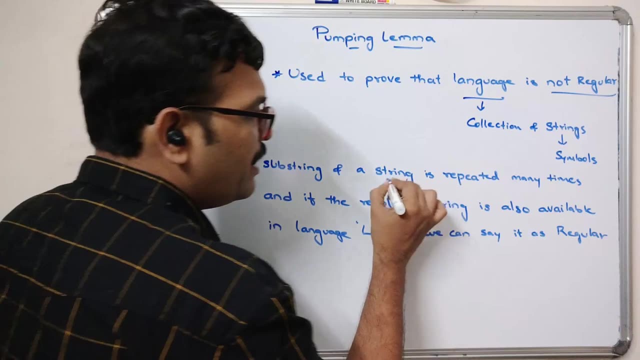 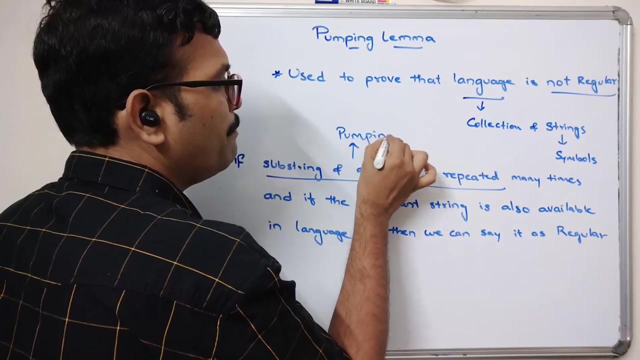 string is repeated number of times and the resulting string is also available in the language, then we can say it as a regular. So this is the pumping lemma And repeating the string. that means repeating the substring. this is called pumping, And lemma means that is nothing. 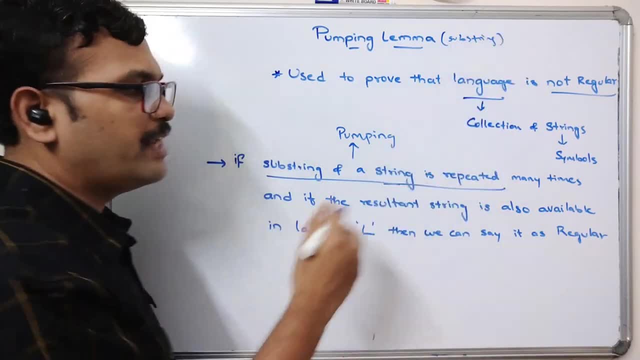 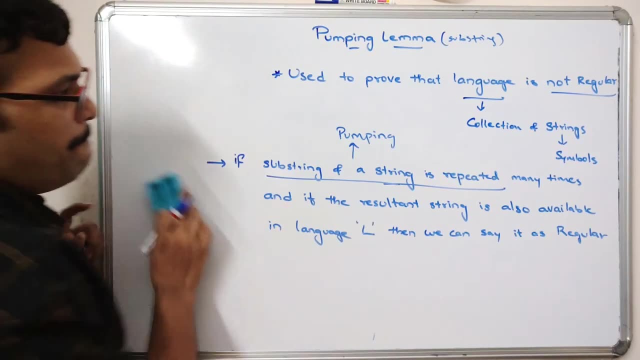 but a substring, right. So if you consider any substring, that must be repeated many times so that the resulting string should be also in language L. So we will prove that, okay. So before going to this one, it should satisfy the three constraints, right? So first one, 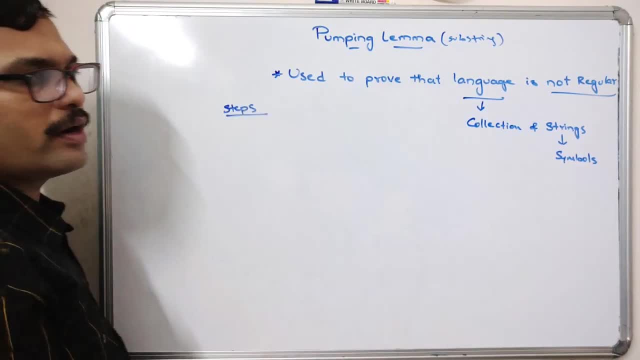 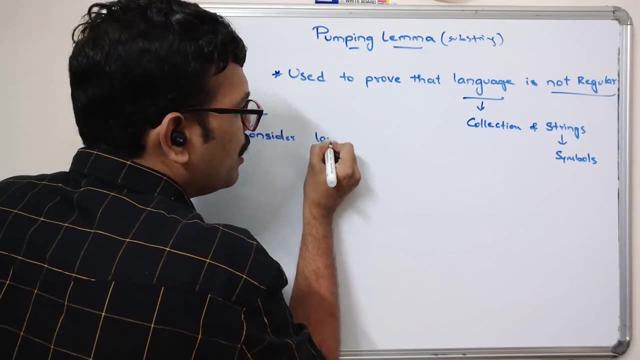 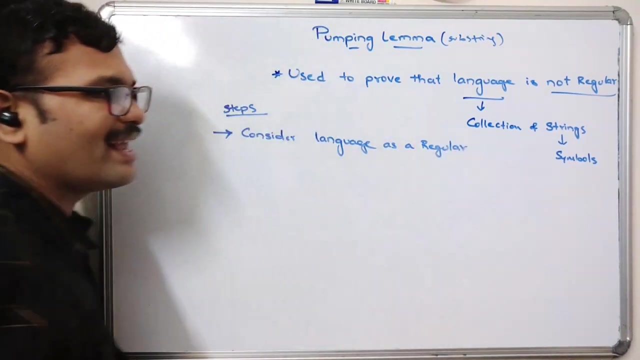 the steps required are in order to prove that language is a not regular. the first step is consider language as a regular. So first we need to consider that language as a regular and we need to prove the contradiction. And the second one and the second point: 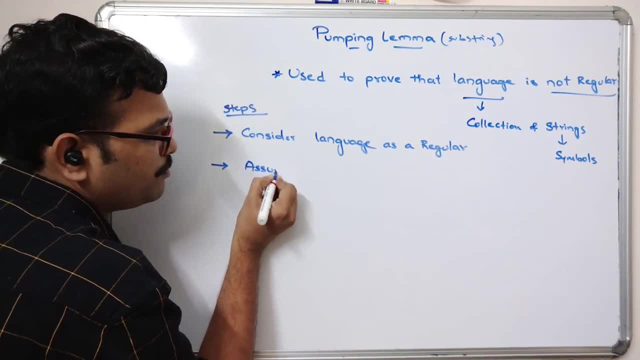 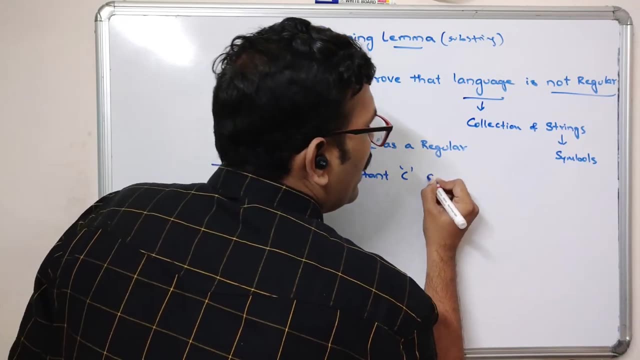 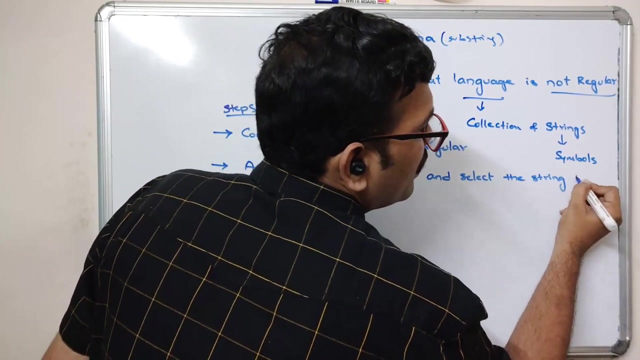 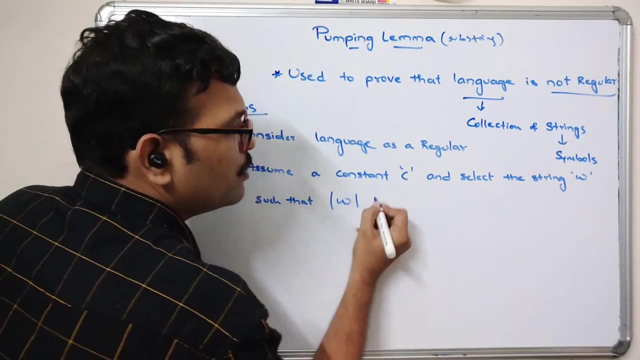 so assume a constant C, a constant C, and select the string W such that mod W must be greater than or equal to C. So we need to. leads to the next point. So this is the first point. So we need to. 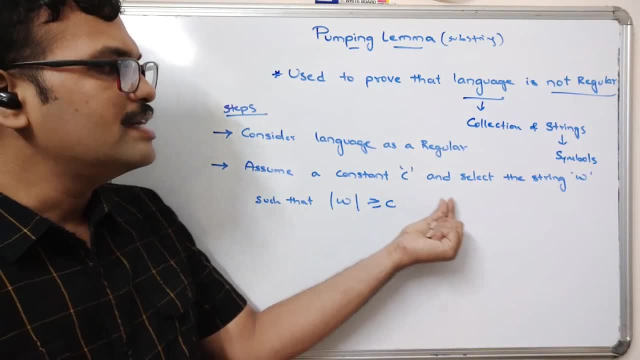 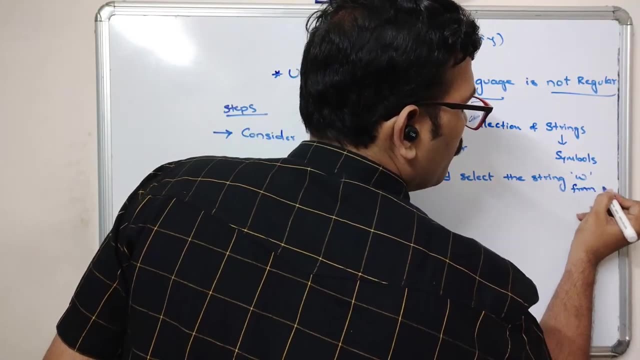 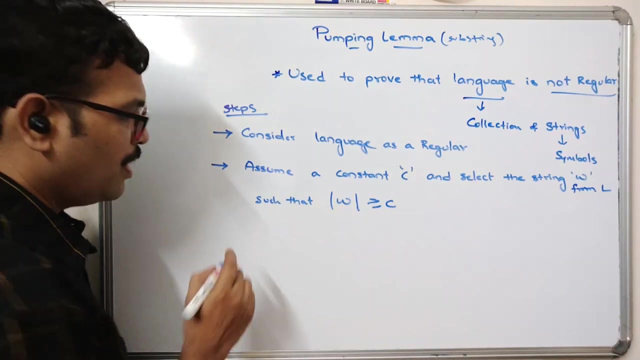 consider some constant C, C as a constant and select the string W from the language. select the string W from L, that means from language, such that the length of the string should be greater than or equal to particular C. And the next one after selecting this. 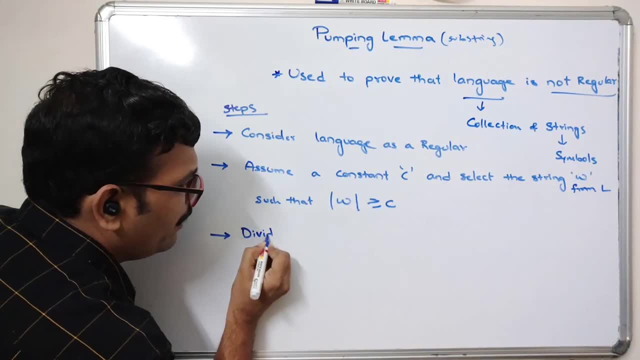 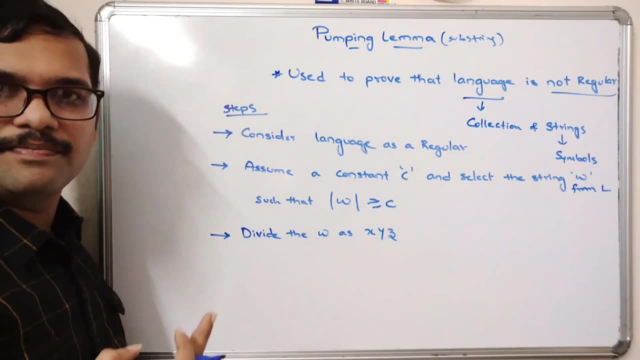 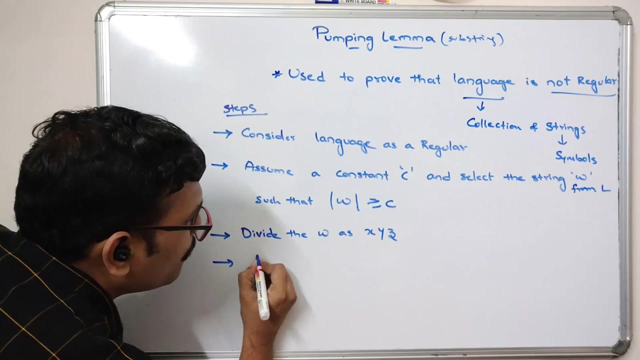 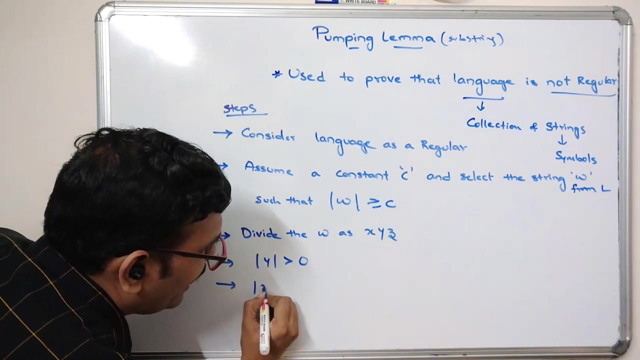 W. so divide the W as X, Y, Z. that means the three strings. So we need to divide the W- that means complete string- as three substrings, such that mod Y should be greater than 0, so mod X, Y should be less than or equal to constant C. 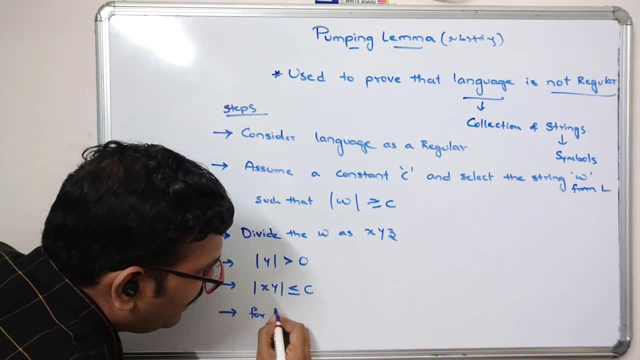 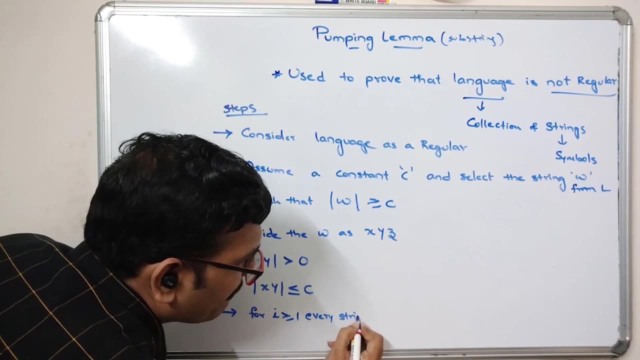 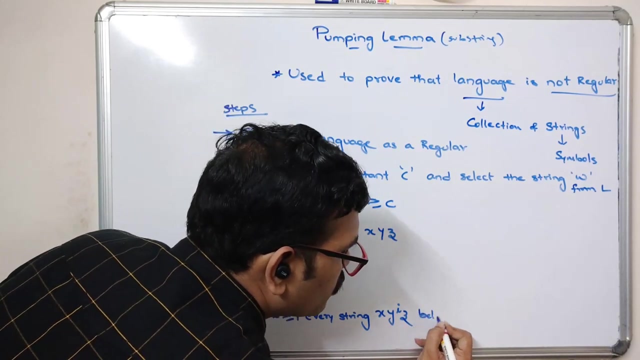 And the third one: after selecting this W, we need to divide the W as X, Y, Z. that means the third constraint is for I greater than or equal to 1, every string, every string of the form X, Y, power, I, Z must be, belongs to L. L means language, right. So here we. 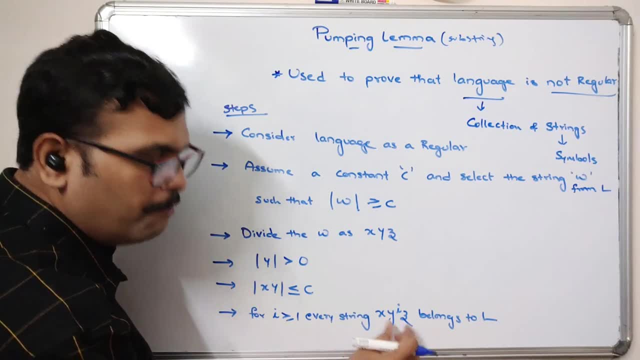 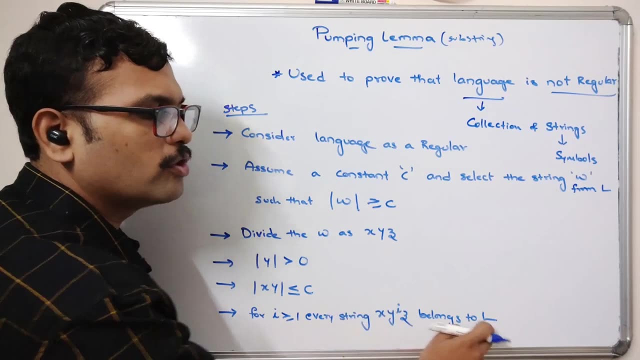 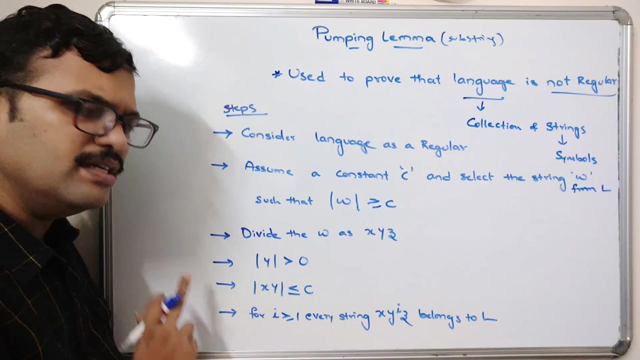 are just repeating the substring Y multiple times. So that is what we have done. So I greater than or equal to every string of X, Y power I, Z should be belongs to L. Then we can say that the grammar is a regular If any one of the constraint is violated. 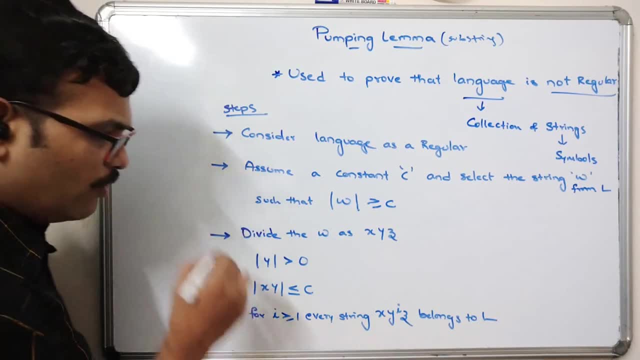 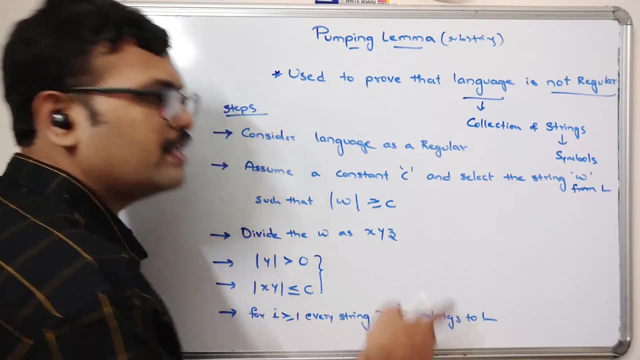 automatically we can say that language is not regular, So automatically we can divide the string into X, Y, Z by satisfying these two conditions. And if this condition is also satisfied, then only we can say: the grammar is a sorry, the language is a regular language. 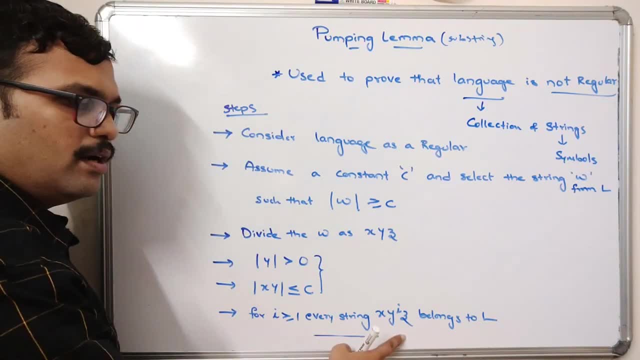 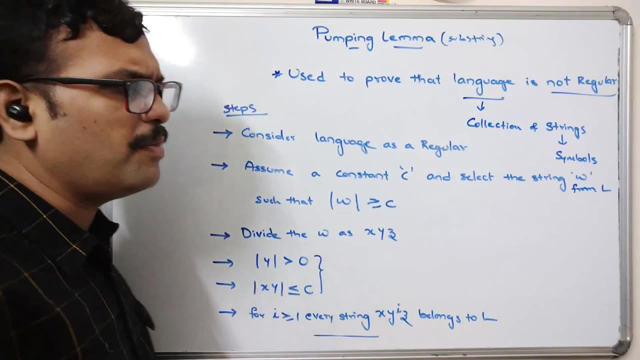 And if this point is not satisfied automatically, we have to prove that. I mean, we can say that the language is not regular. So we can take one example and we sort out right. So just remember this one: First, consider the language as a regular and write down the language first. 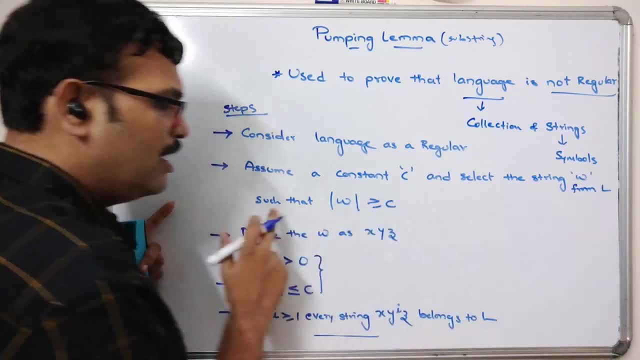 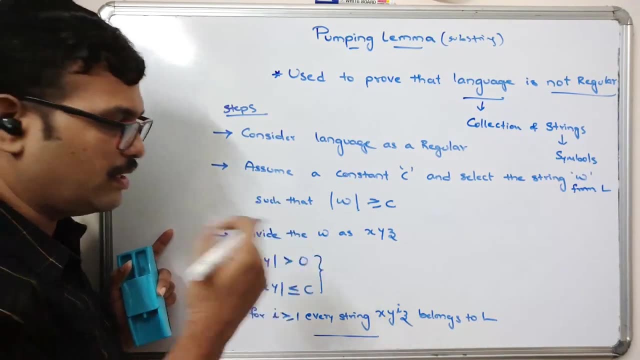 and assume a constant C and select the string W from L such that length of the string should be greater than or equal to C. And we need to select that particular string which is greater than or equal to C And next divide the constraint. So we have to divide the. 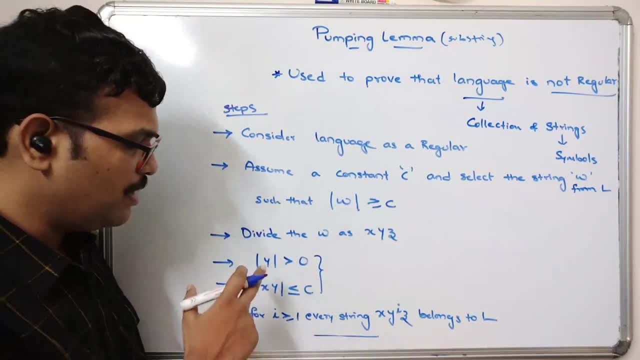 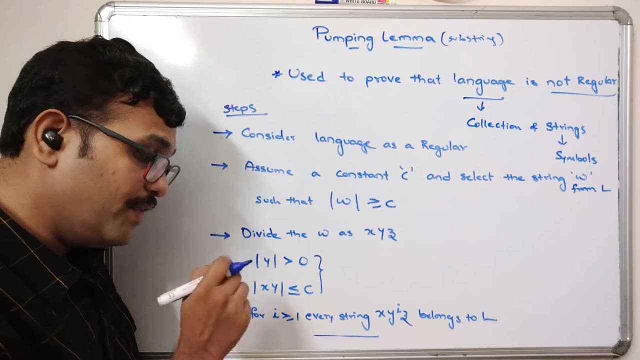 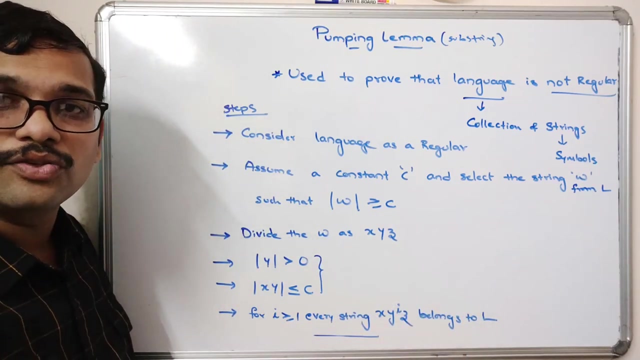 complete string as X Y, Z. that means the three parts, such that the length of Y should be greater than 0, length of X, Y should be less than or equal to C, And for every I value greater than or equal to 1, the string X Y, power I, Z should belong to L. So then, 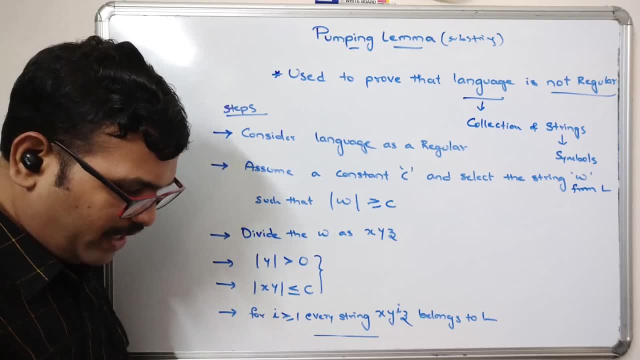 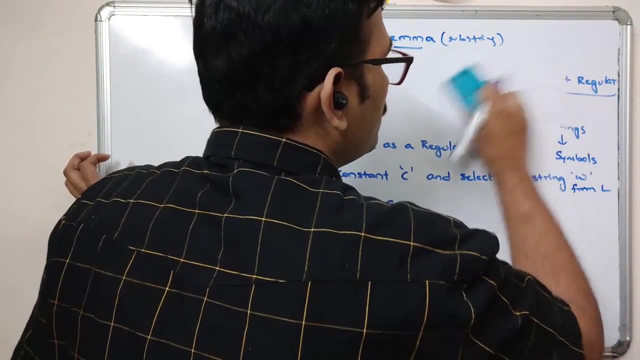 only we can say that the language is regular. Now we will take an example, We will consider an example. So once again I am saying: this particular pumping lemma concept is a regular. concept is used to prove that language is a, not a regular. So contradiction right. 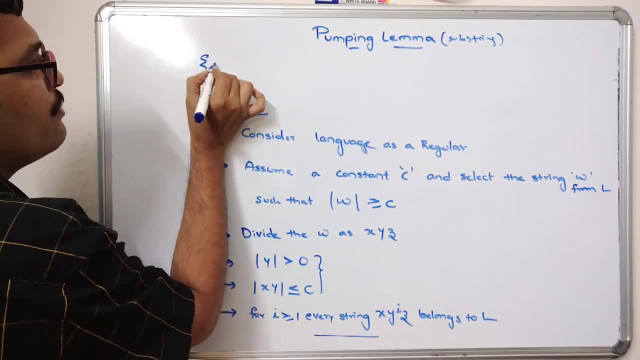 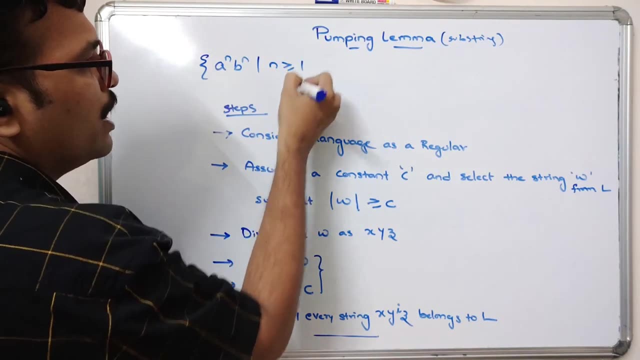 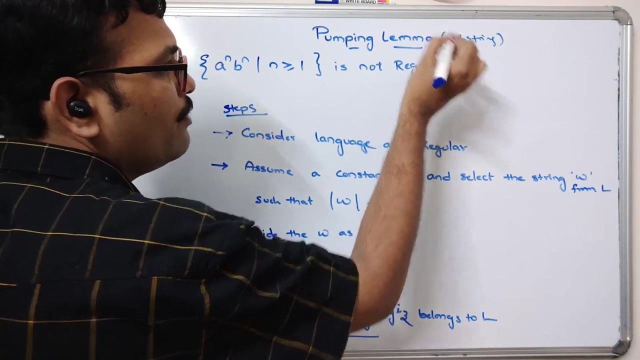 Now. so consider the language: A power N, B power N, where N greater than or equal to 1, okay, is not a regular. We need to prove that it is not a regular, So we will have- I mean, we will be getting the questions like the language will be given and we need to. 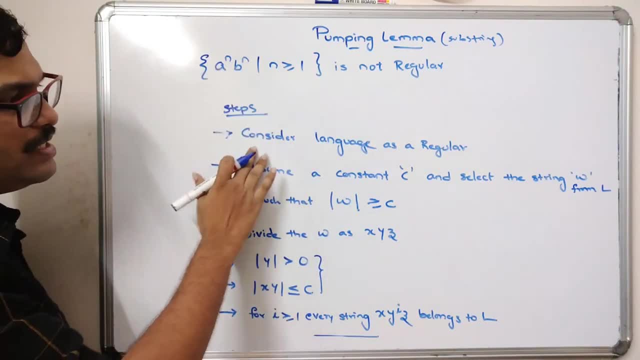 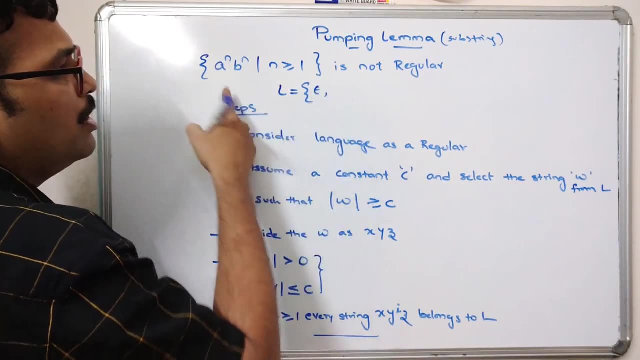 prove that this language is not a regular, First consider the language as a regular. So consider the language L. So what are the possibilities? So epsilon, right and C, we can simply write it as 0, right. So 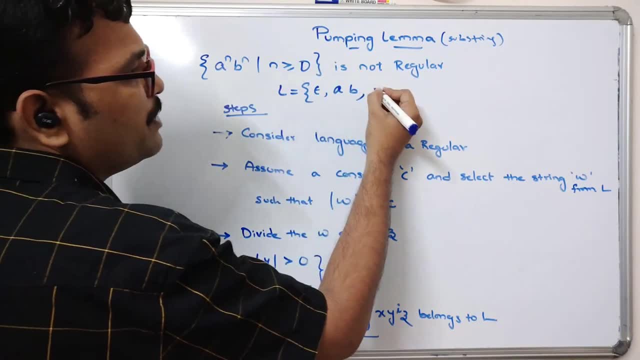 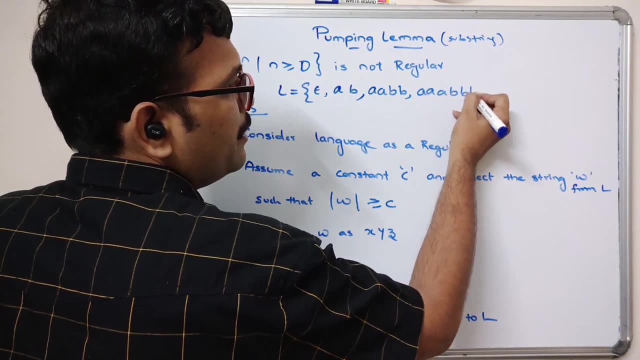 if it is 1,, it will be A, B. If it is 2,, A square, B square. that means A A, B, B. And if it is 3,, A, A, A, B, B, B. If it is 4,, 4 As followed by 4 Bs and so on, That means number of parts. So that means A A, B, B. So that means A A, B, B. So that means number of parts. So that means number of parts. So that means number of parts, So that 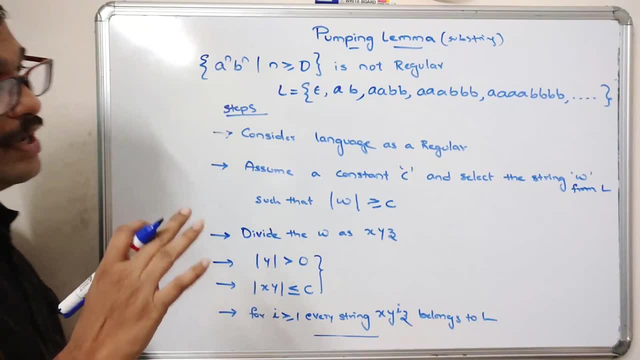 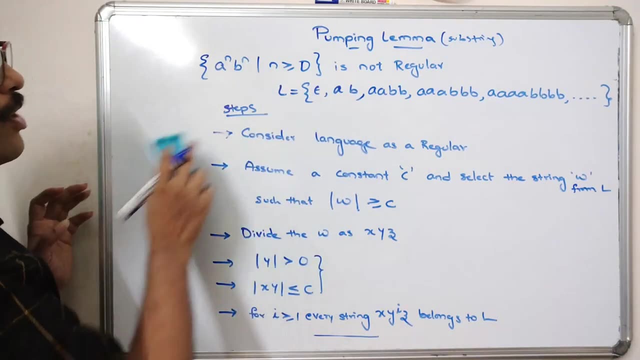 means number of As, followed by number of Bs and the- I mean the equal number of As and Bs- should be there. Equal number of As and Bs should be there right Now. we have considered this one. Next, assume the constant C and select the string W. So I will select the. 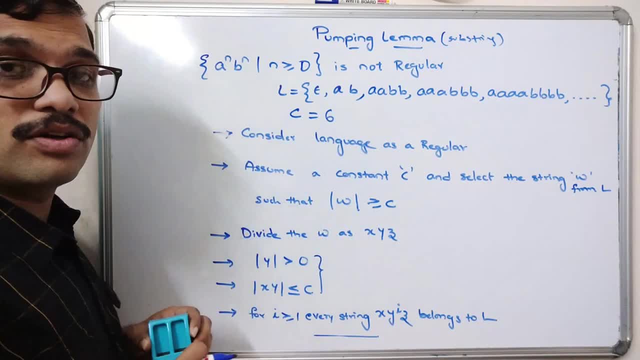 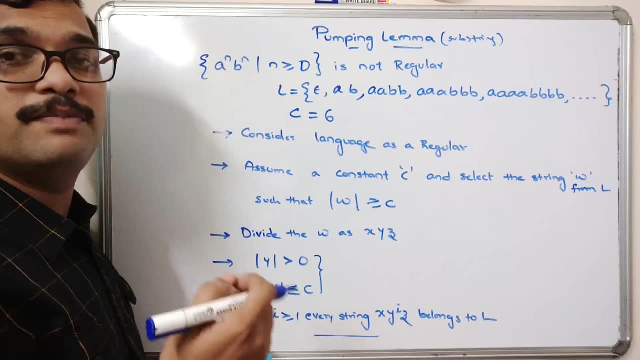 constant, C as some, 6,, 6 as a constant. So I need to select one string from the language whose length is greater than or equal to 6.. That means the minimum length must be 6.. So I can consider the strings from here. 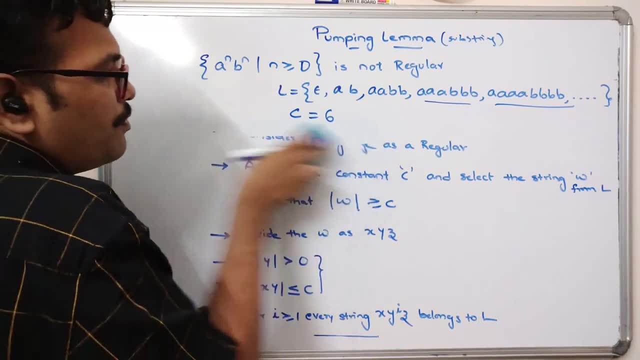 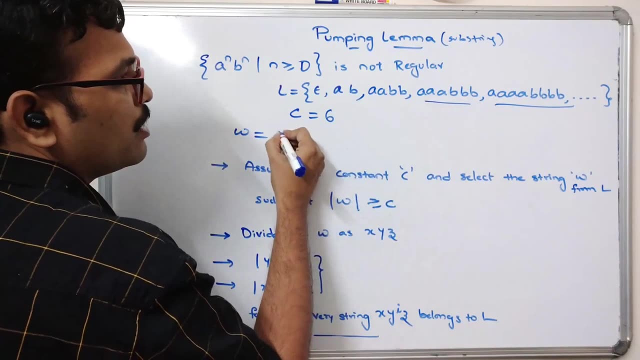 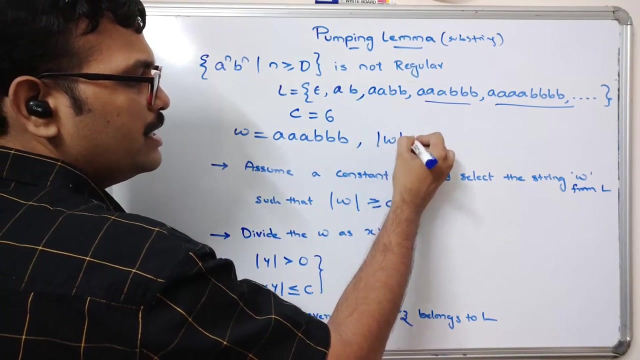 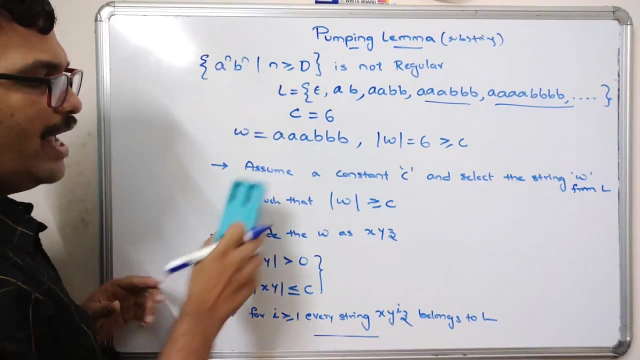 So I can consider the strings from here itself. right Now I am just erasing this one, So I will consider the W as this one: A, A, A and followed by 3 Bs. That means here the length is 6, which is greater than or equal to C. right Now, assume a constant C and. 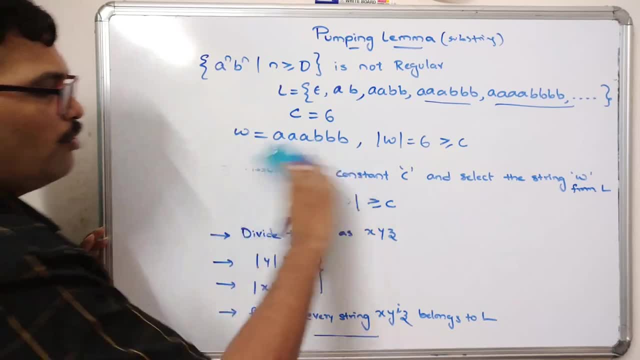 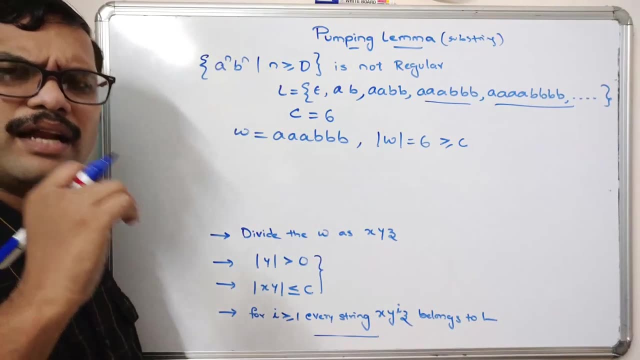 select the W. So I have selected this W. Now, after this step, what we have to do? We have to divide this as a X, Y, Z. You can consider any substance, any combination, right, So you can divide in any way. So I will. 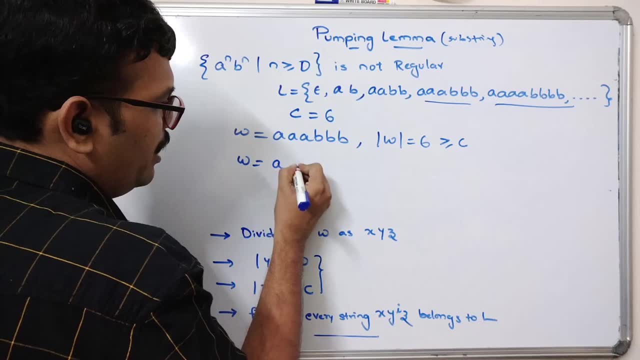 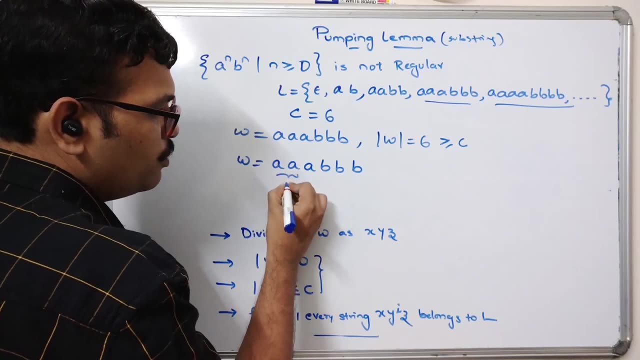 take this one. So W is equal to A, A, A, B, B, B. So among this one, I will consider this 2 as X, this 2 as Y and this 2 as Z. So this is not a fixed set. You can also. 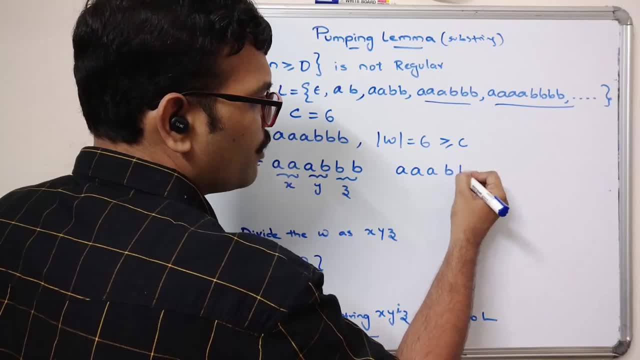 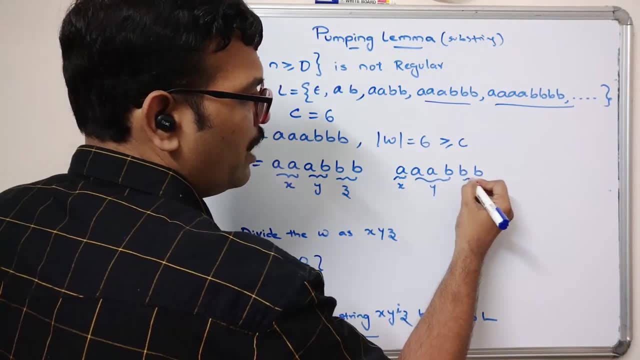 consider… Sorry, there are a lot combinations. You can consider lot of combinations, but all the 3 conditions should be true. So if you consider this one as X and this one as a Y and this one as Z, You can consider this one also right. So you can consider any combination. 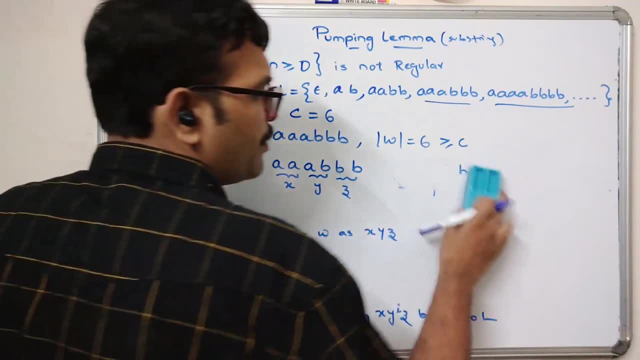 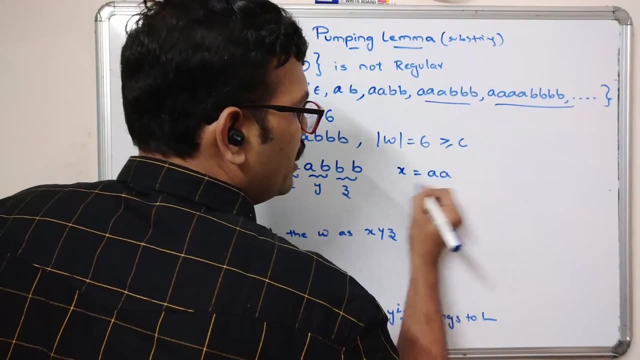 You can consider any combination, So I will consider this one. Okay, I will consider this one Now. X is A A. X is equal to A A. Y is equal to A B, Sir, No, sir. 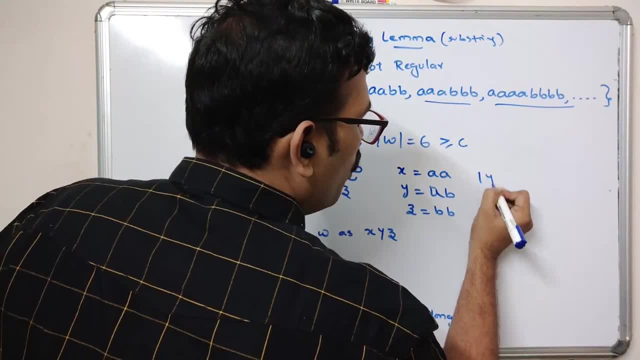 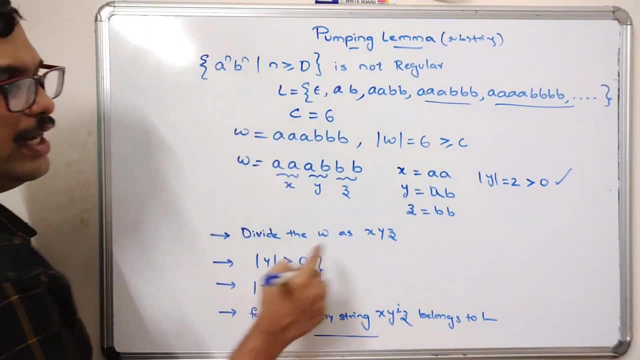 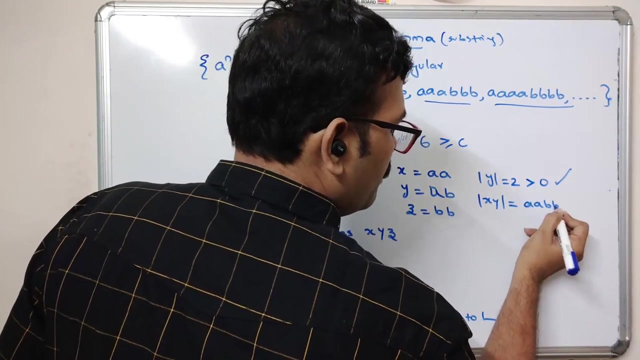 Sir, Erase, Erase, And Z is equal to B, And here you can observe mod: Y is equal to 2, which is greater than 0. Condition 2.. So this condition is 2.. Right, And next, X and Y is equal to A, A and B, B. 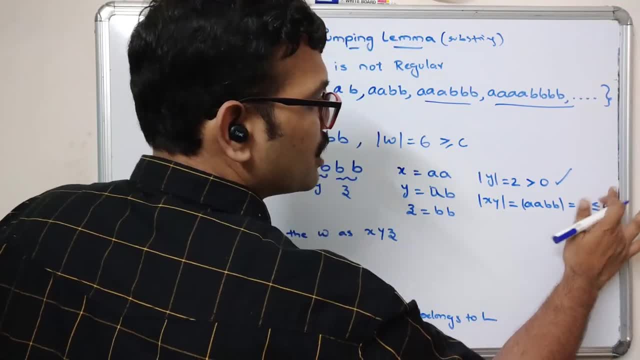 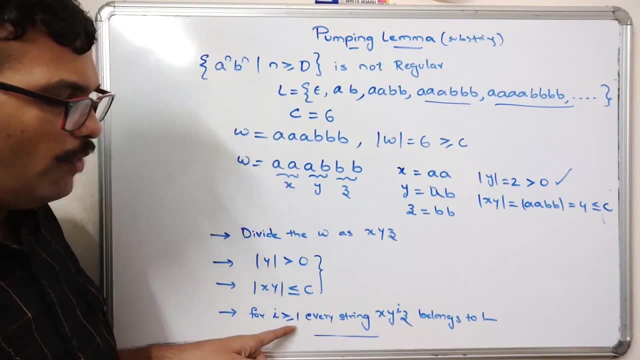 Which is of length 4, which is less than or equal to 6 or C. Simply we can say it as a C. Right, So this is also 2.. Now we need to check the third one, For I is equal to 1, every string X, Y, power, I, Z belongs to L. 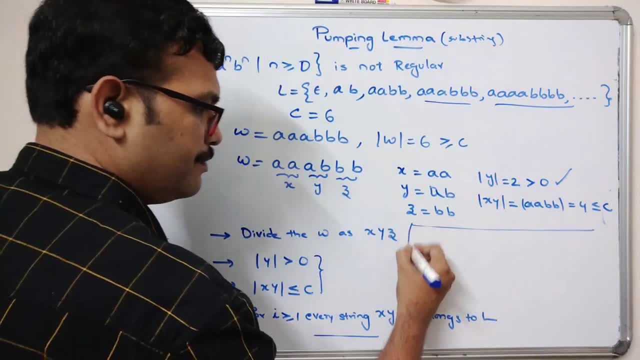 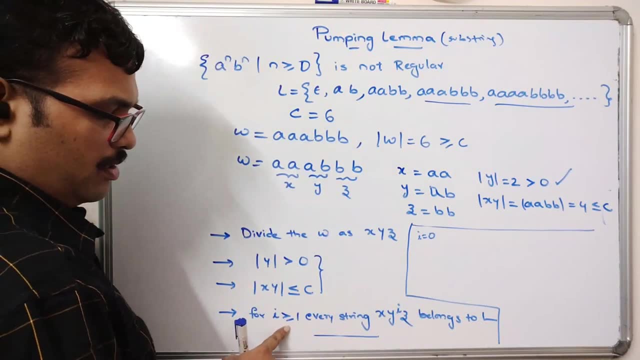 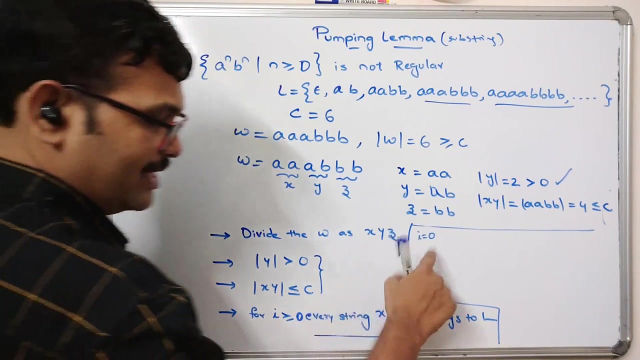 Now you can see here the third one. The third one. So if I becomes 0.. OK, So we can simply consider 0.. OK, I greater than or equal to 0.. So if I is 0.. X, Y, power, 0.. 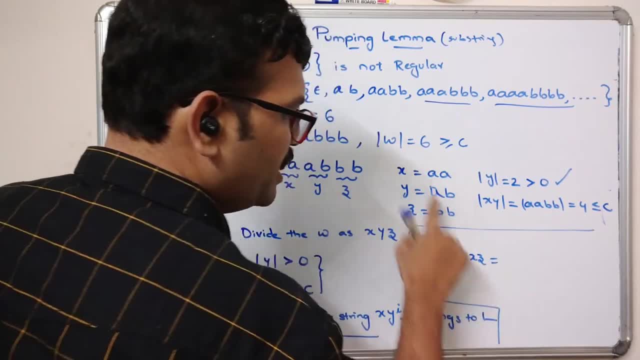 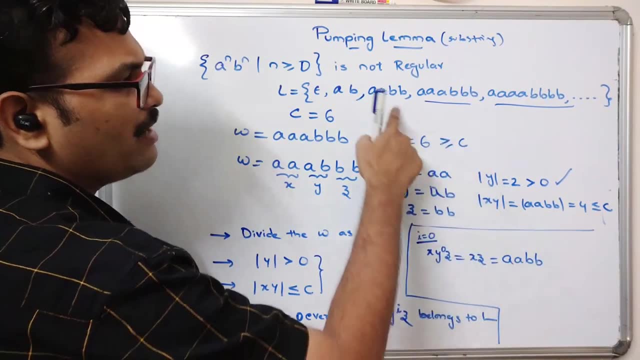 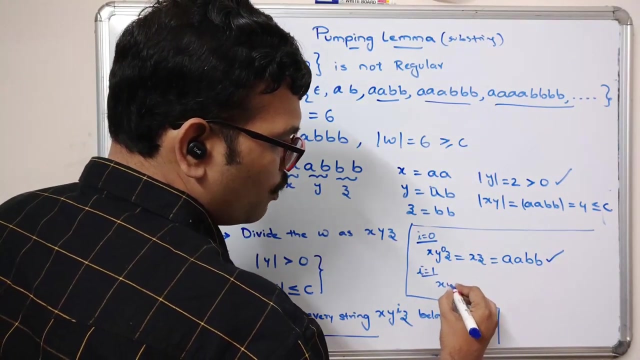 Z. That means X Z. OK, X Z means A A and B B. So is it a possible string available in the language? Yes, This is true. Now I becomes 1.. So X Y Z, which is nothing but A, B. sorry, 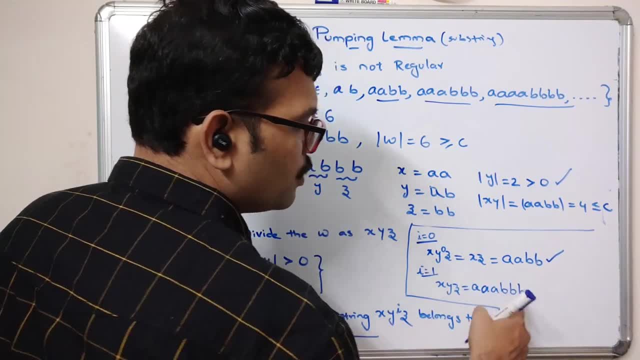 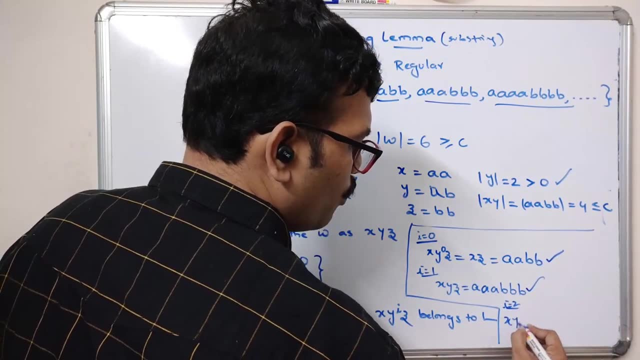 A, A, B, B, B. So this is also available in this string. Yes, Now consider I is equal to 2.. Then X Y square Z, X Y square Z. So here Y power 1, Z, Right. 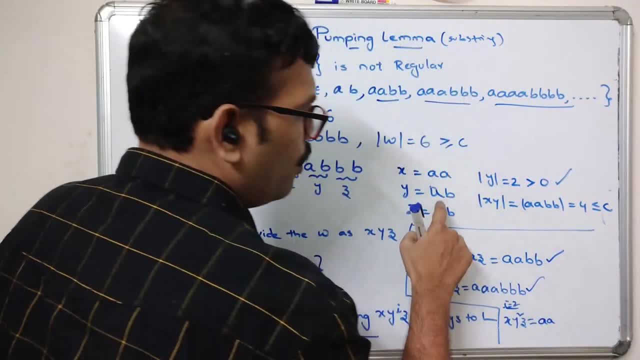 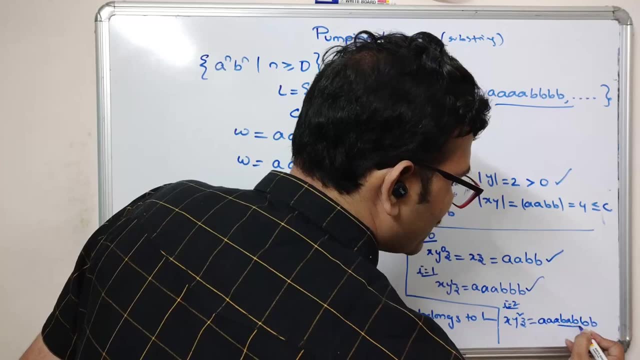 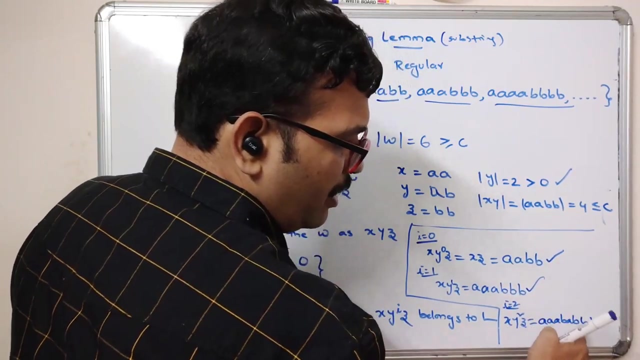 X Y square. Z means X means A A, Y means A, B, A, B, Z means B, B, Because this is X square Right, So we need to write the Y term multiple times. Now you can observe A, A, A, B, A, B, B, B. 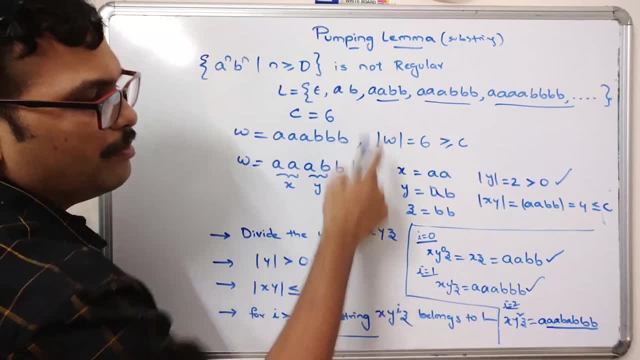 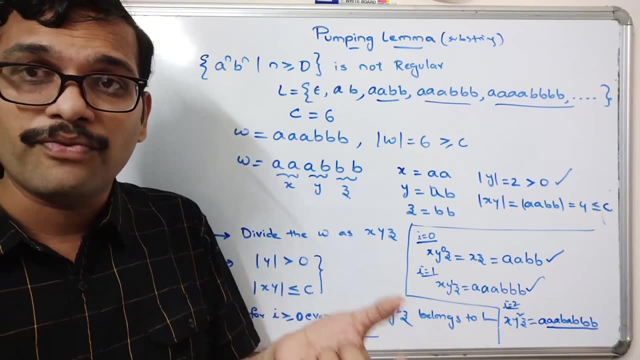 So here this is not available in our language, Because our language consists of the multiple number of A's followed by multiple number of B's, And the number of A's and B's should be equal. So here also the number of A's and B's are equal. 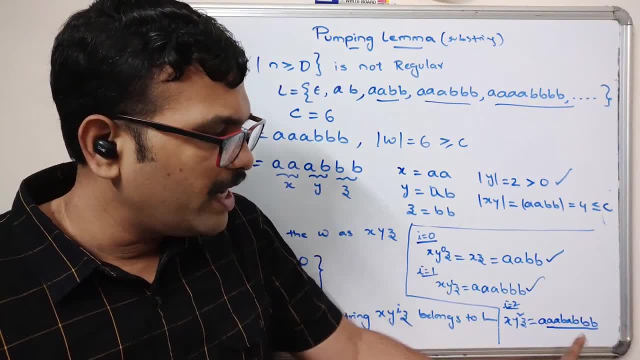 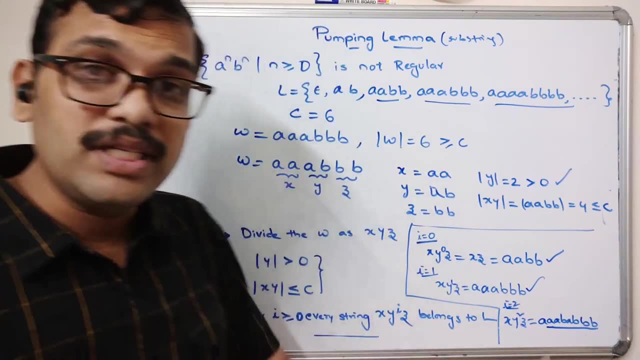 But so the number of A's is not followed by B, Because, see A, 3 A's are there, followed by B. Again we are getting A, Again we are getting B. So this is completely wrong. And this is this string is not available in this language. 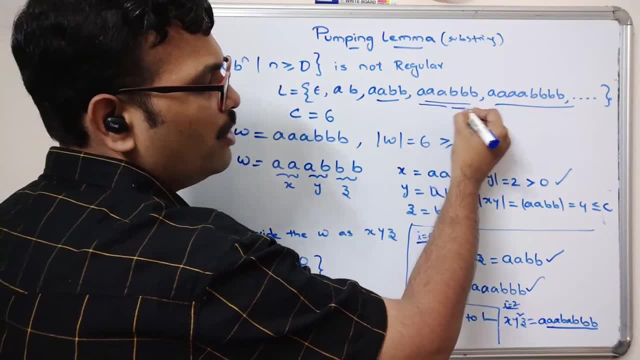 Right, Right, Right, Right, Right, Right, Right. So this is completely wrong. So here also we can observe A's and B's. So here also we can observe A's and B's. Then only you have to get the number of B's. 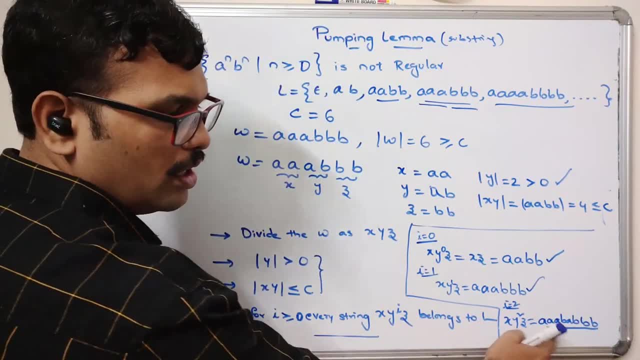 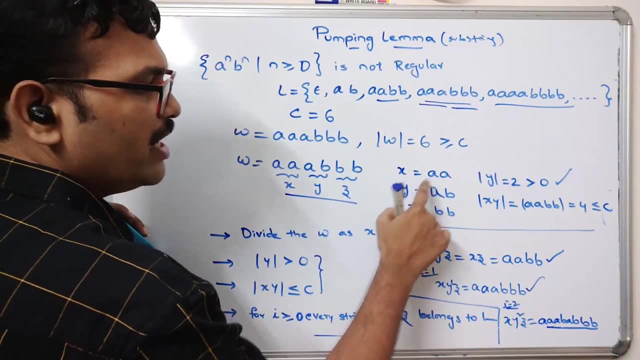 So, but here, after B, again, we are getting A. So this is not a valid string. Okay, It's not a valid string. So if you consider this one, So X is equal to A, A, Y is equal to A B, Z is equal to B- B. 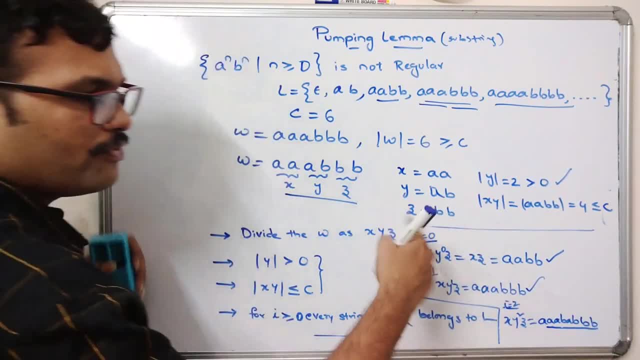 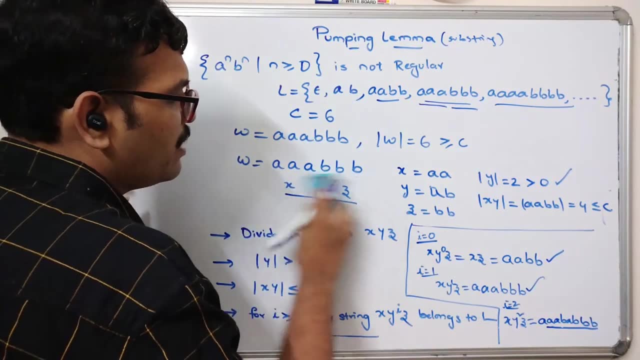 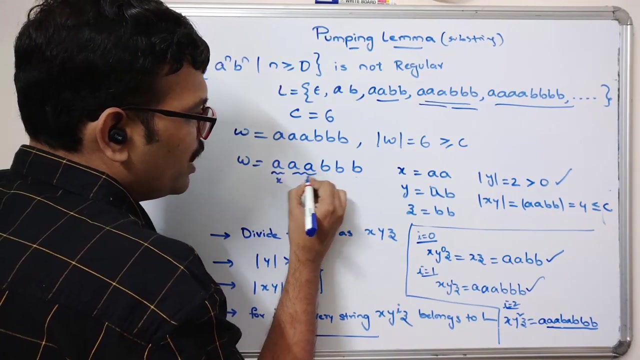 We are getting that. the repetition of the string is not available in language, But now you just change the pattern. So X Y Z. You change the X Y Z. So let us take the this one as X, this one as Y and this one as Z. 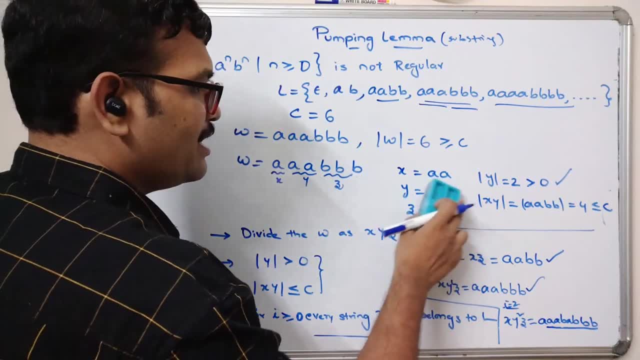 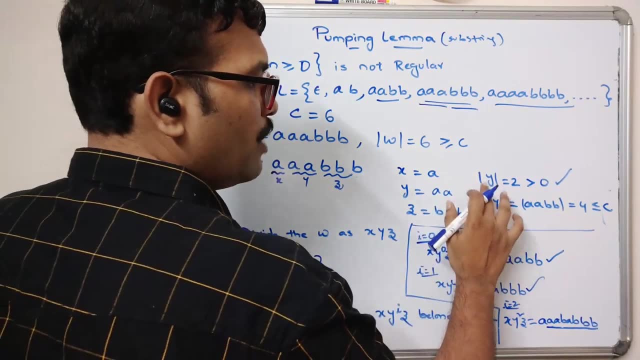 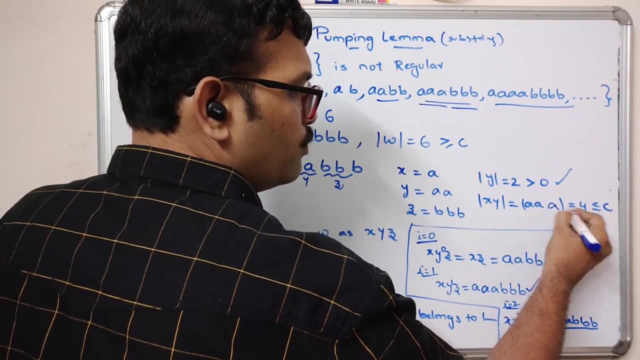 Okay, Now you can observe here: X is A and Y is A, A and Z is B, B. And you can observe here: Y is equal to 2, that is greater than 0.. X and Y is A, A, A, which is nothing but a. 3, which is also less than or equal to C. 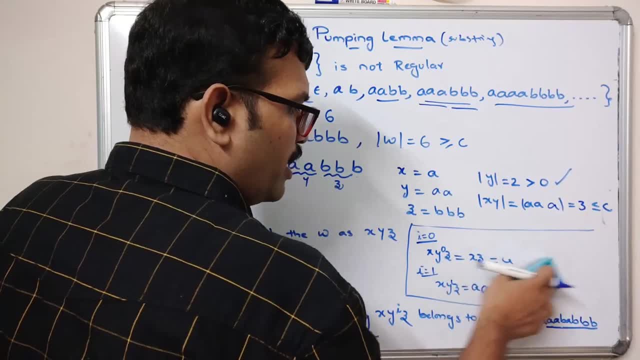 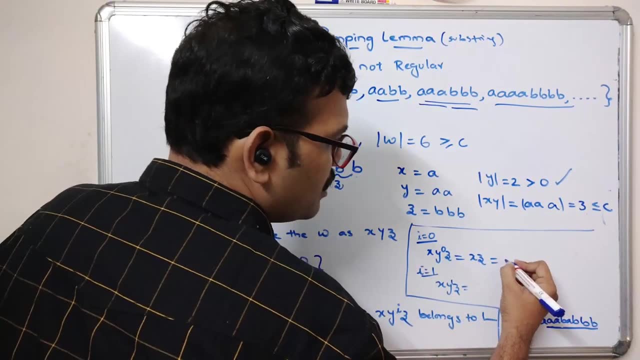 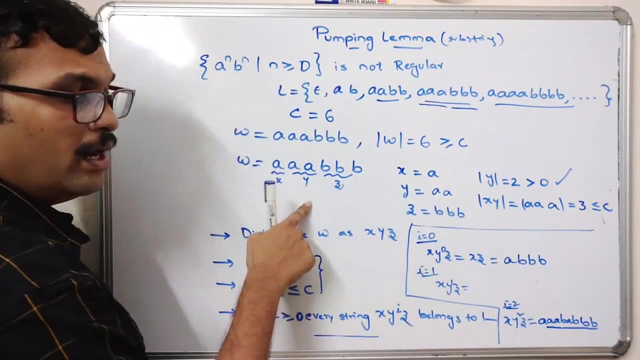 Yes, True. Now simply, you can observe here. So for X is equal to 0, X and Z X, Z means A, B, B, B, X, Z, A, B, B, B, according to this one. 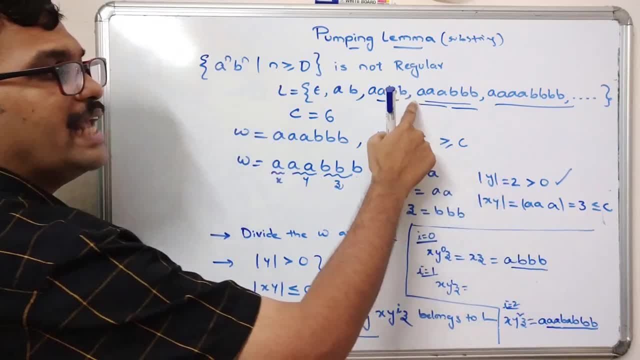 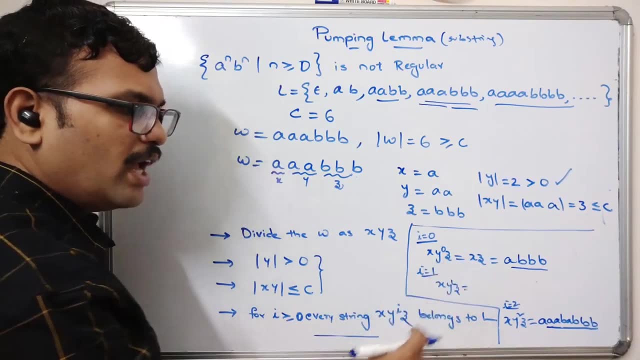 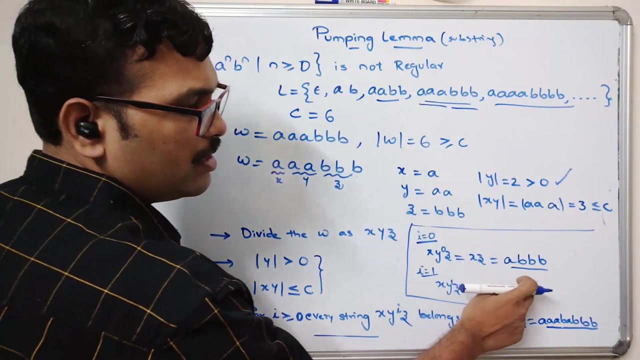 Right And simply, you can say: this string is not available in L language, L, Right. So just remember, we are taking the substring Y and we are just recursively called the Y. We are calling that Y, such that the resultant string should be available in L, But here. 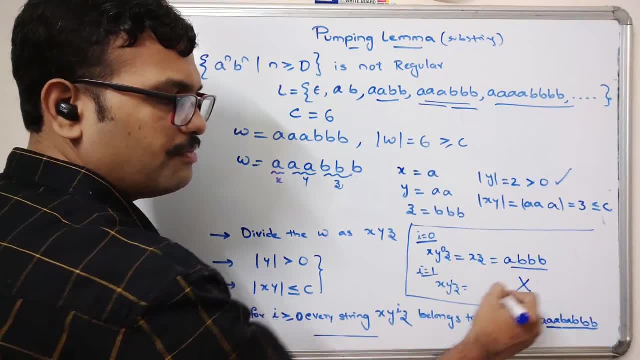 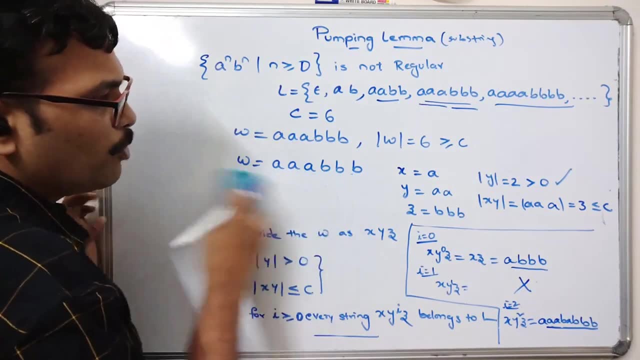 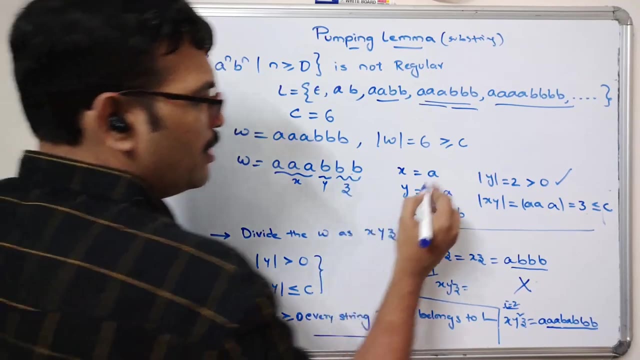 it is not available in L, So that again, this is false. That means language is not regular. Now we can select one more pattern. We can select one more pattern. So simply, you can select X as all, As Y as B, and Z as B- B, So all As are in X and 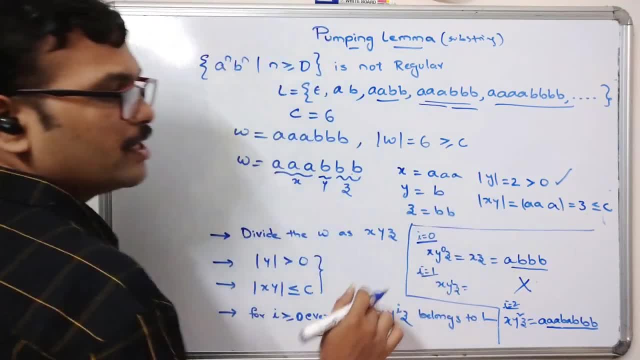 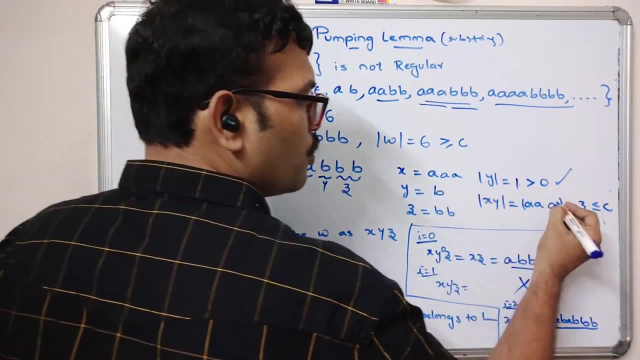 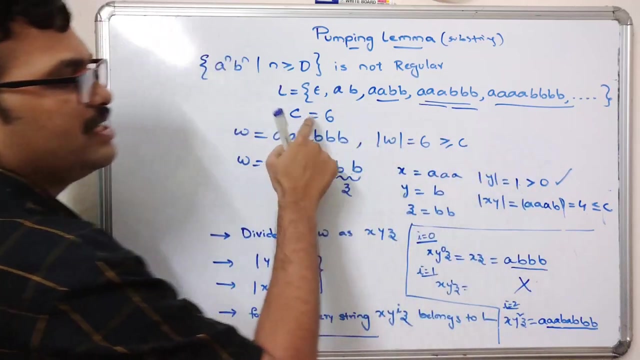 Y with a, B, single B, and Z is B, B. Now you can see. So mod Y is 1,, which is greater than 0,, 2, and X in Y. So A, A, A and B, So which is nothing but 4, and less than or equal to C, C is 6 here. 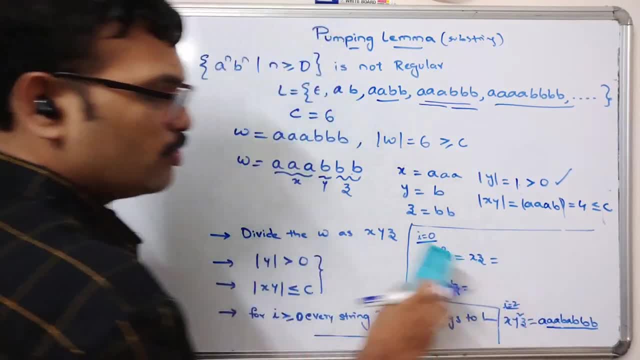 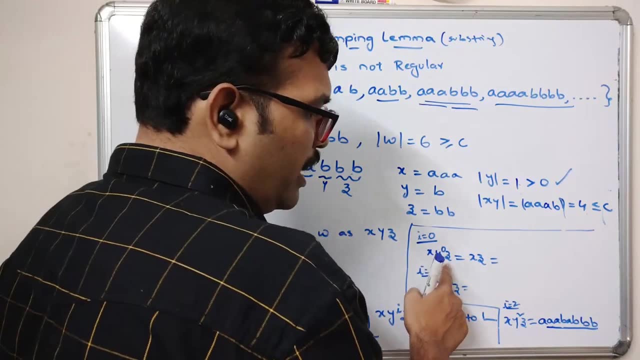 Right Now you can observe If I is equal to 0, if I is equal to 0, so remember, I greater than or equal to 0,, not greater than or equal to 1.. Right, So, I is equal to 0,. X and Z. X and Z means A, A, A and followed by B, B. So here you.